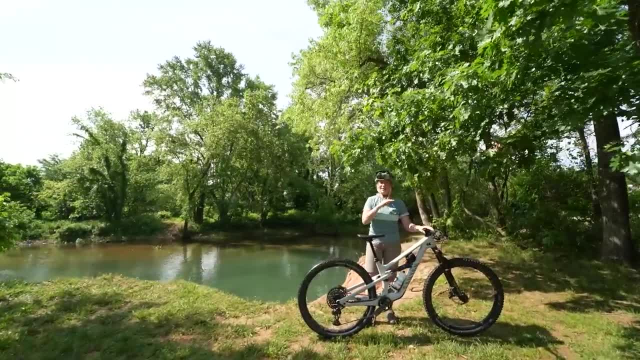 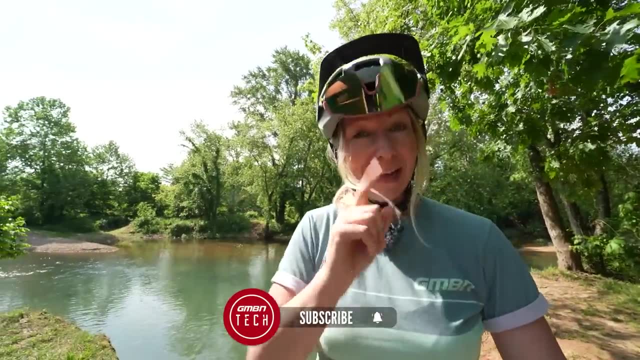 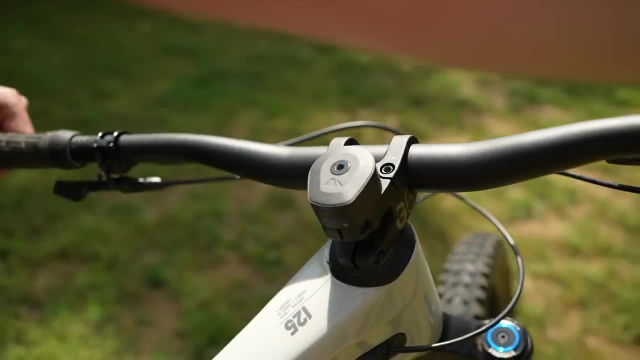 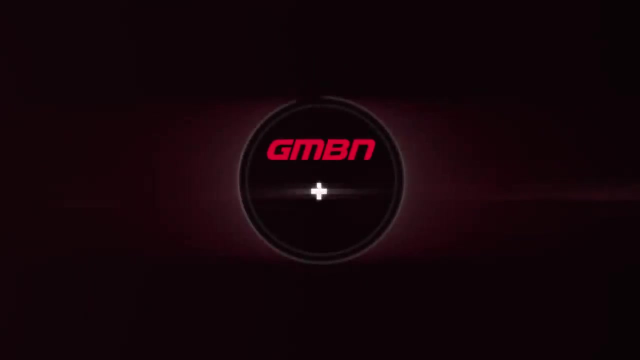 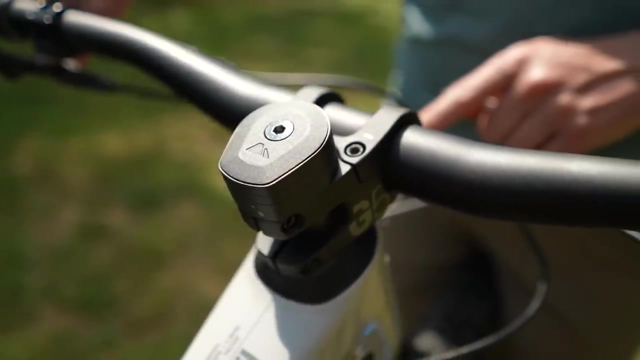 Here are five basic maintenance skills that absolutely every mountain biker should know how to do. So stay tuned, because they're so simple and if you're new to the channel, hit subscribe. So if you feel a knocking at the front end and you've checked your axle so that your wheel is 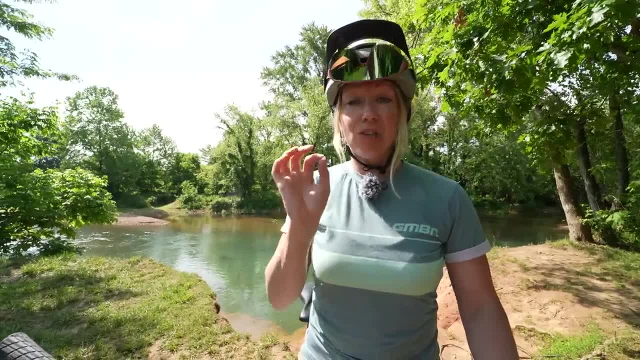 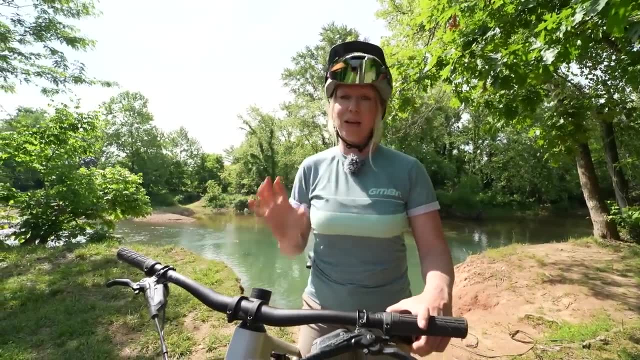 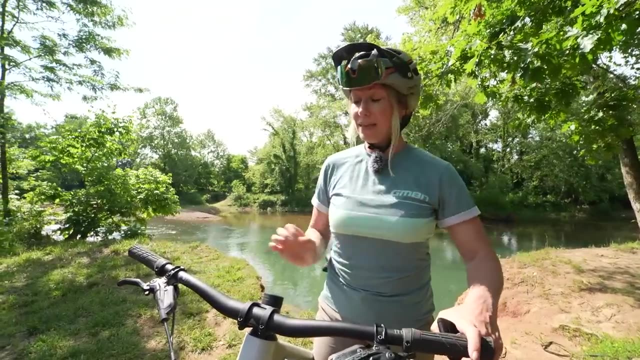 definitely insecure and that wheel's not wobbling, then chances are it's a loose headset, and it is quite common and all it is is fiddling with tightening of bolts. so it's really simple Now to diagnose the problem and make sure you actually do have a wobbly headset. all we need. 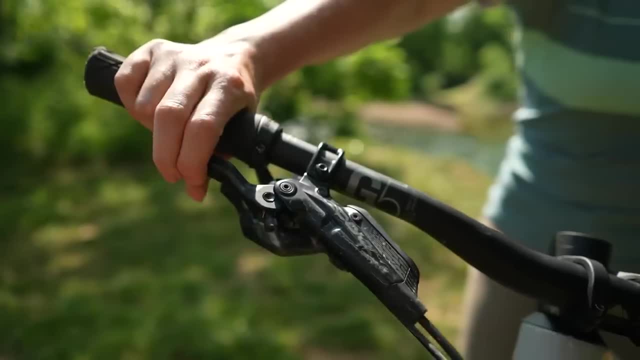 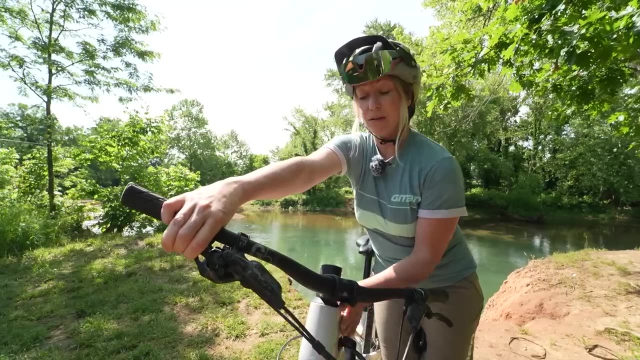 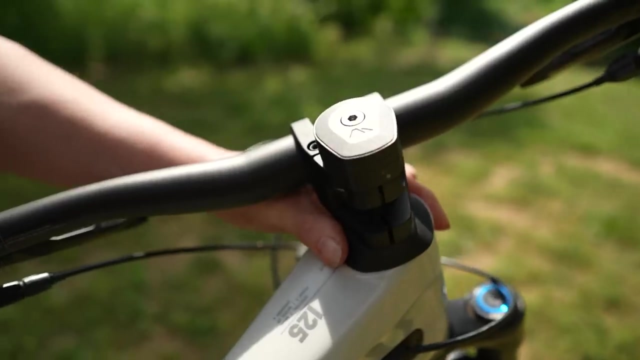 to do is turn the bars, apply the front brake and rock your bike. You can even hold on to the headset area around here at the top of the frame. give it a rock and you probably will feel it wobbling in your fingers. So we know that's a headset problem. 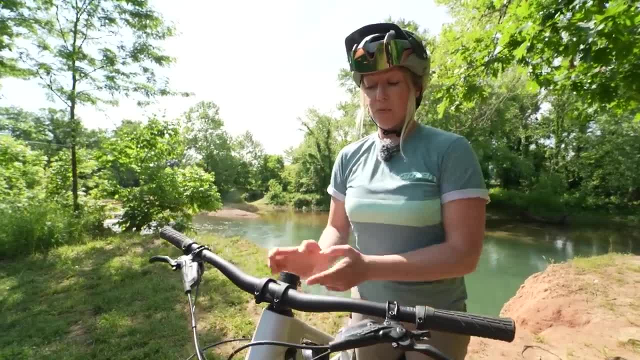 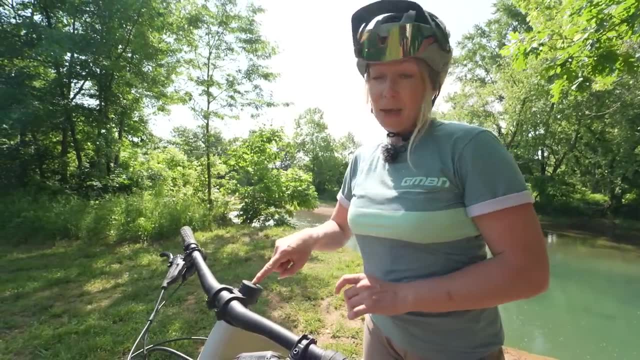 and what you're going to need to do is loosen up the bolts on your stem, because that's clamping to the steerer tube of your forks. Loosen that up and to tighten the headset, it's the bolt right at the very top. So you're going to need some allen keys, a little bit of a hammer and a little bit of a. 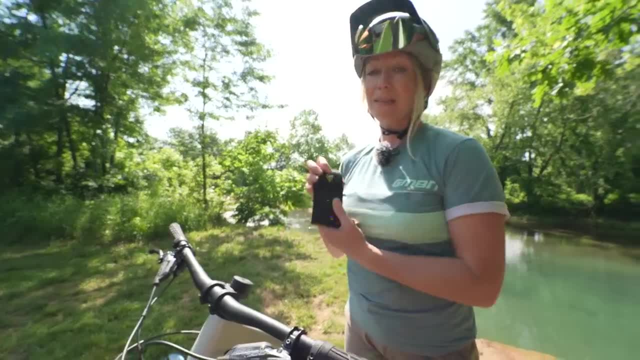 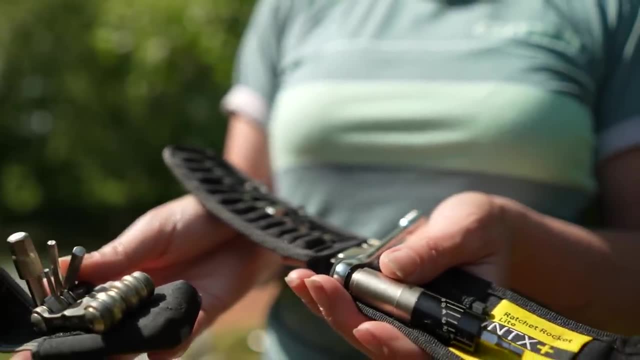 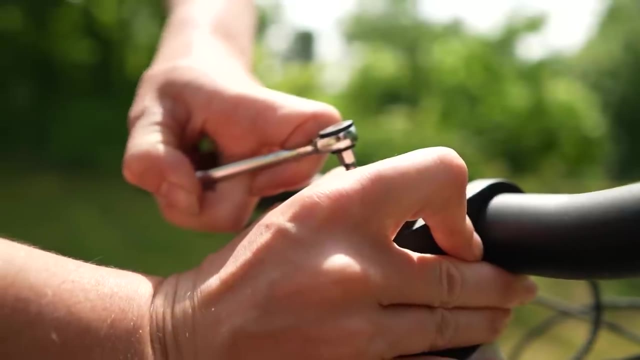 wrench or you're going to need a multi-tool like this, better still, a torque wrench or a mini torque ratchet system like this- and all you need to do is tighten up that bolt to about four or five newton meters, which is kind of gentle hand tight if you're not using a torque wrench. 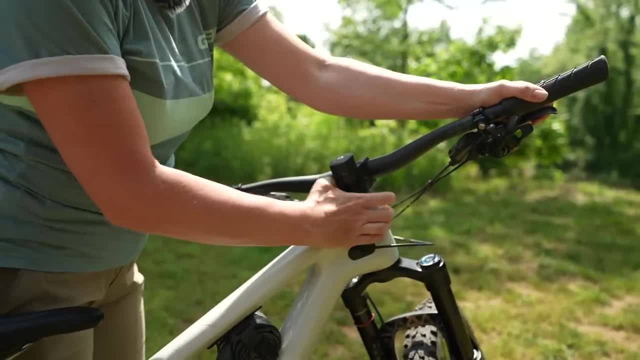 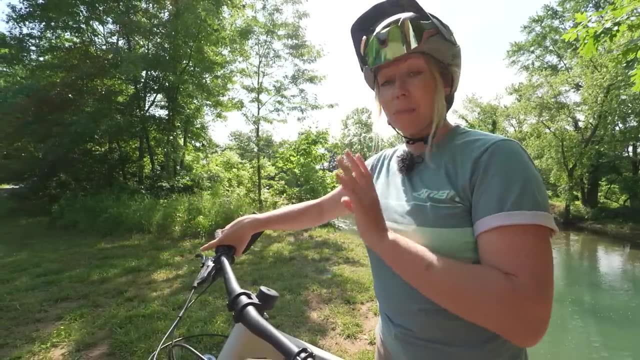 and then try rocking it again. I know your stem is loose, but that's fine. Try rocking it again, and if it doesn't wobble and it doesn't knock, then you've secured it in place. If it doesn't wobble and it doesn't knock, then you've secured it in place. 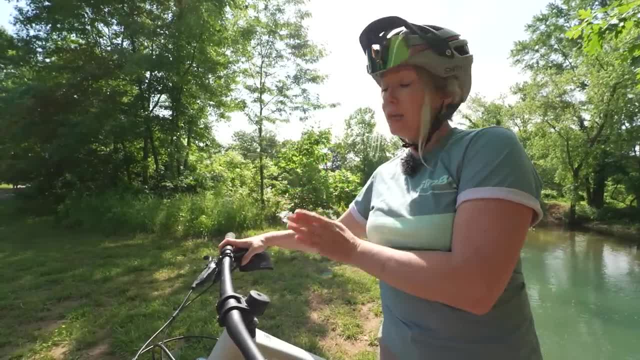 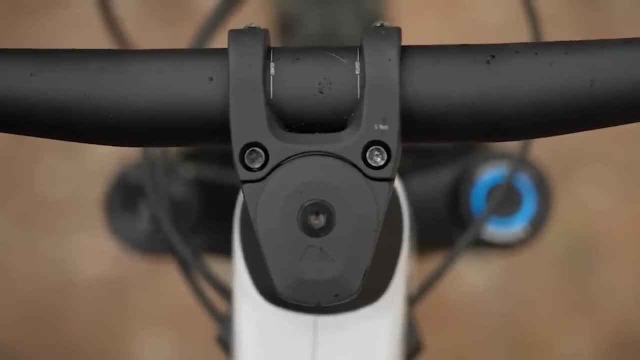 Try rocking it again, and if it doesn't wobble and it doesn't knock, then you've secured it in place, And then all you need to do is make sure that your stem is aligned with your wheel. perhaps stand at the front and align your handlebars with the crown of your forks and 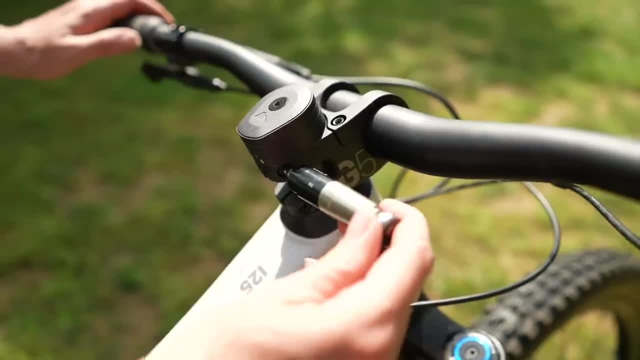 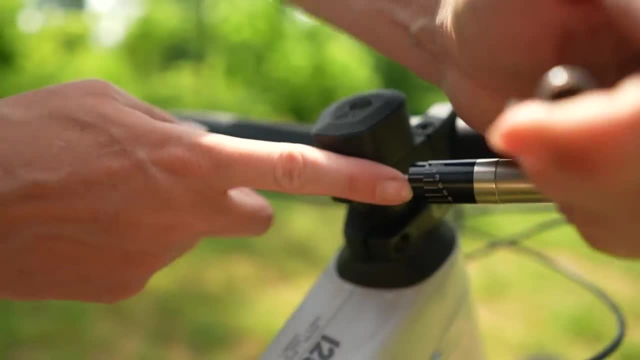 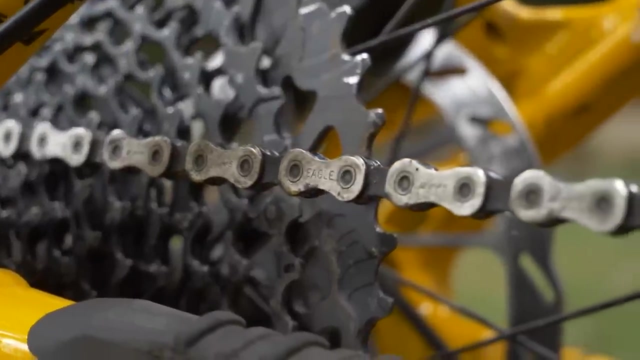 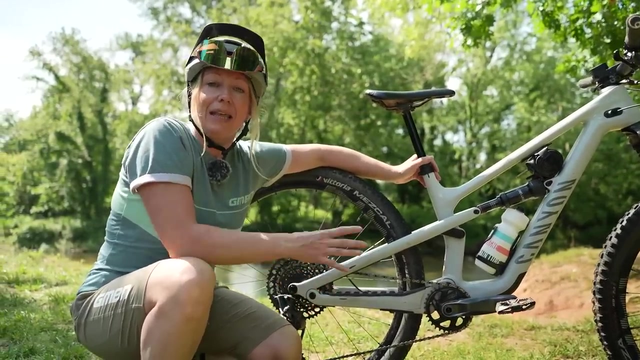 then tighten up those stem bolts again And again. you should be talking to manufacturer spec, usually about four or five newton meters, and you're good to go. The chain is probably the first thing that will wear out on your bike and if you keep on top of replacing this regularly, then it could save you. 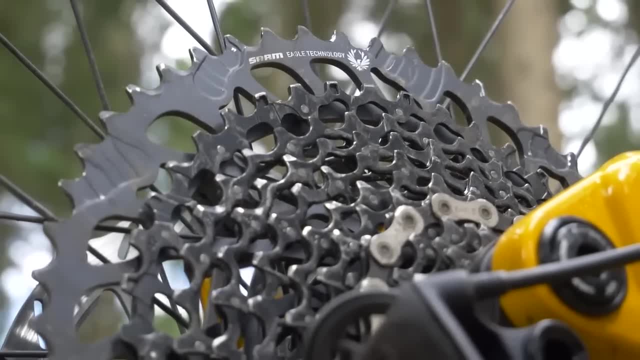 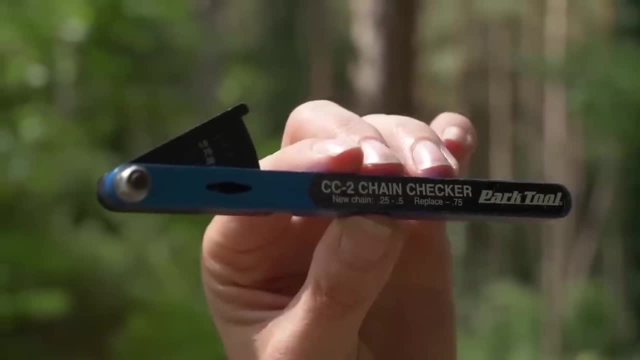 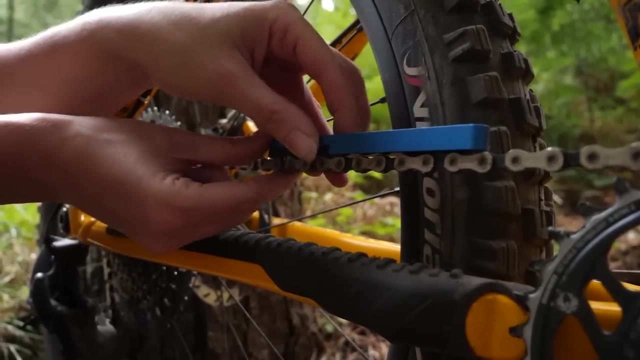 hundreds in replacing cassettes and chain rings, because if you change this regularly, it won't wear these two things out. So what you'll need is a chain checker, and if you've got a 12 speed drivetrain, then changing it around about 0.25 or 0.5 is recommended so that it won't wear out the rest of. 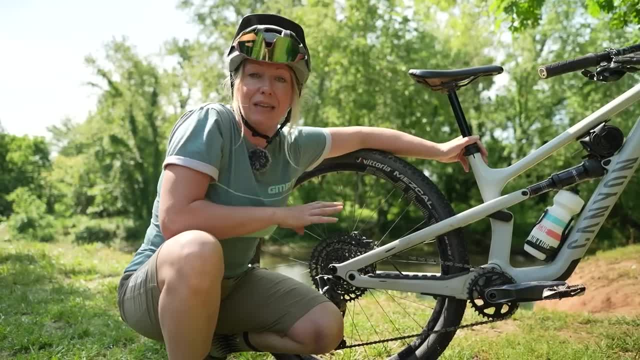 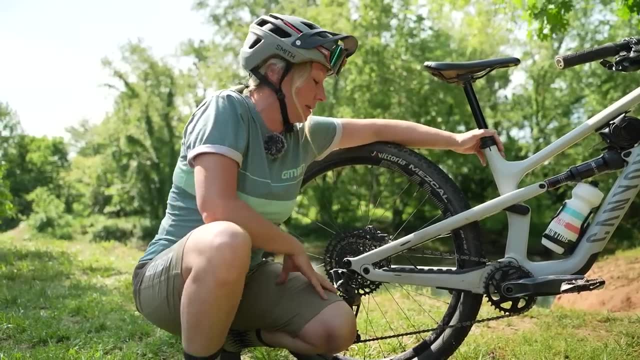 your drivetrain. If you've got a 12 speed drivetrain, then changing it around about 0.25 or 0.75 is recommended. If you have any lesser gears, like 11 speed or 10 speed, you can probably get away with 0.5 to 0.75.. Now to change this it's really easy if you have a quick link. 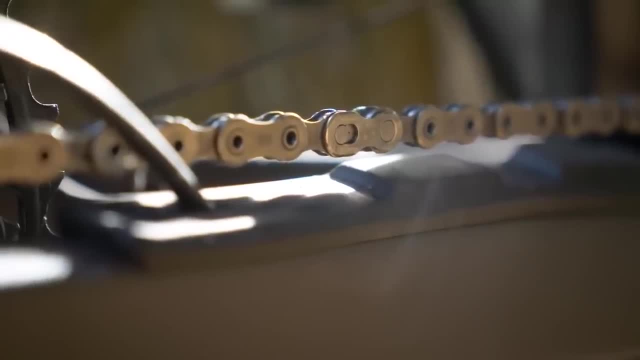 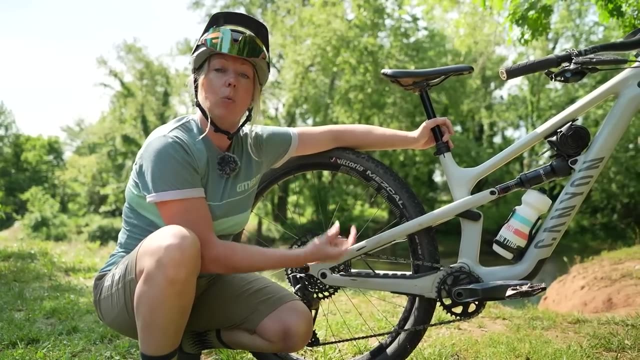 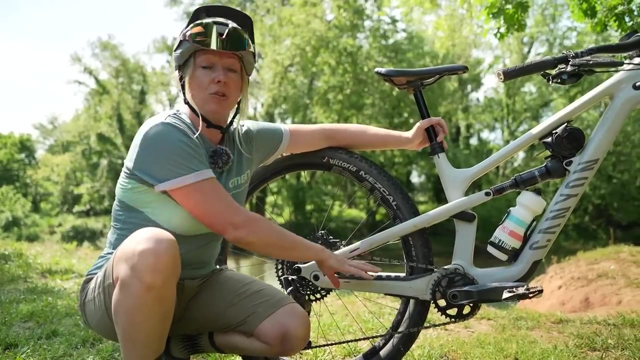 you'll have to find it. it should look like this, and all you'll need is a pair of link pliers, or even a normal set of pliers used at an angle will unclip this link and then, with your new chain, line it up on a table against your old chain and try and match the amount of links used, and then 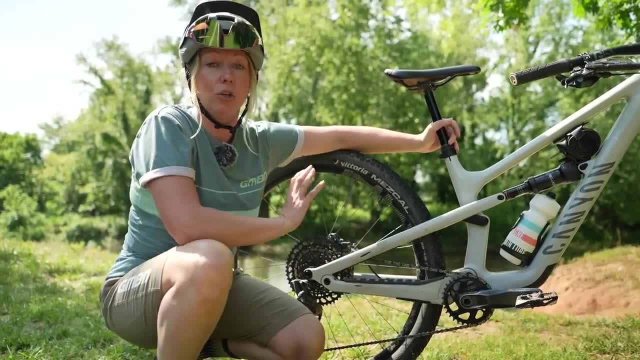 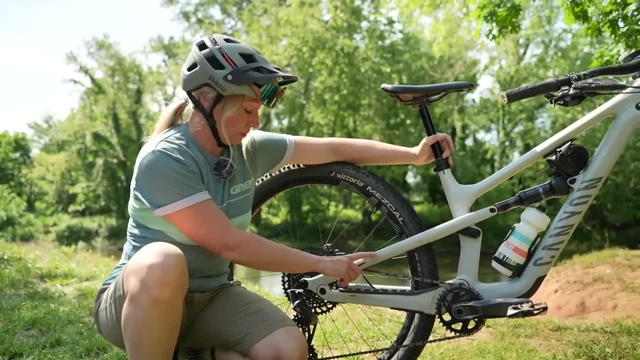 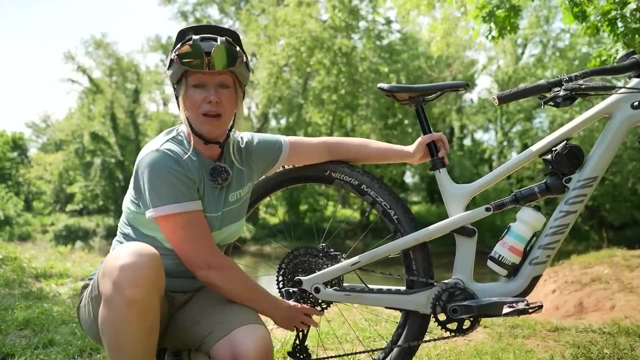 that way, all you have to do is get a new link and attach your new chain. once you've cut it down to length and attach that to your bike. One big tip here is: maybe take a photo of your drivetrain so that you can match how the chain moves around your derailleur and always make sure that it goes behind. 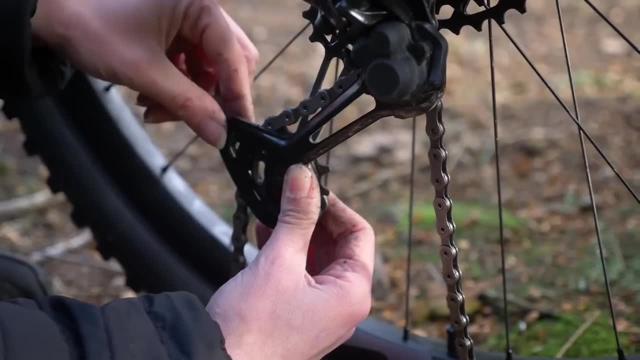 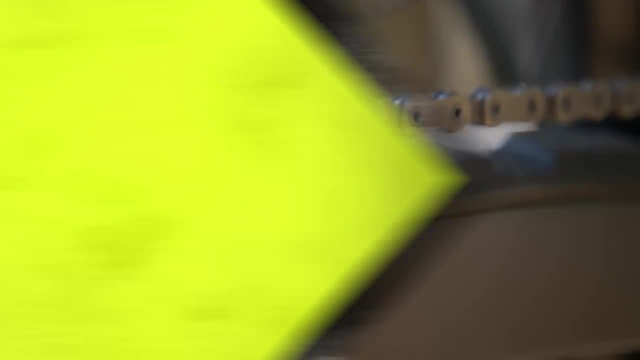 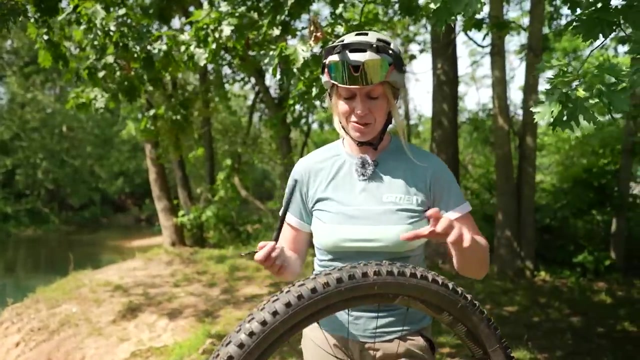 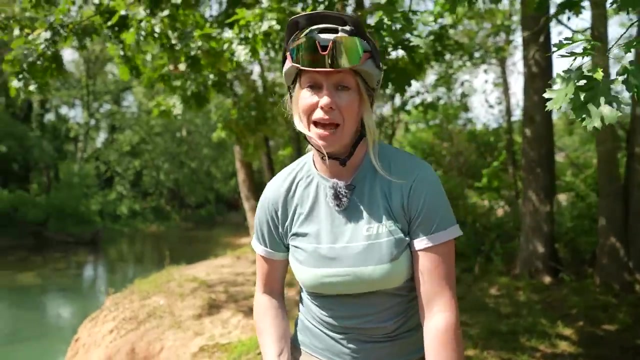 the edge in the derailleur so that it's not rubbing. once you've attached it and your chain is moving, Fixing a puncture is absolutely essential. If you've been relying on other people to help you with puncture repairs on the trail, then now's the time to have a little practice at home, because if 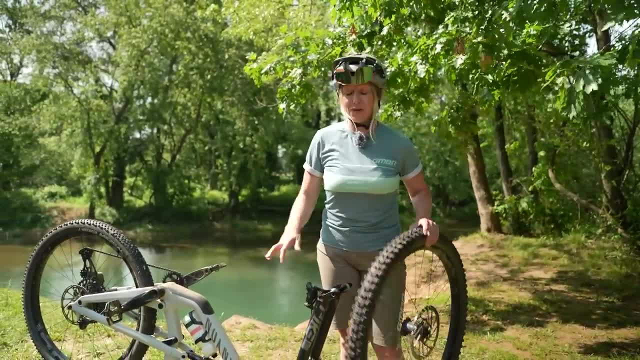 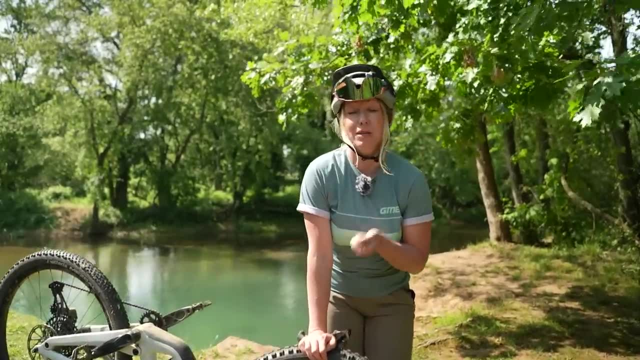 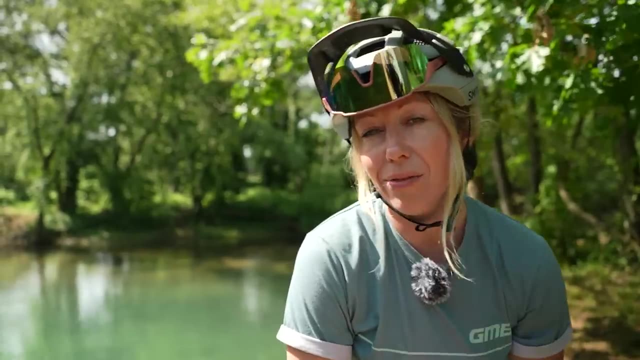 you're ever riding on your own and you get a puncture, it's going to completely ruin your ride. and it's really easy. If you're set up tubeless, then you can use some tire plugs to insert it into the hole and then hopefully the sealant inside will seal around. 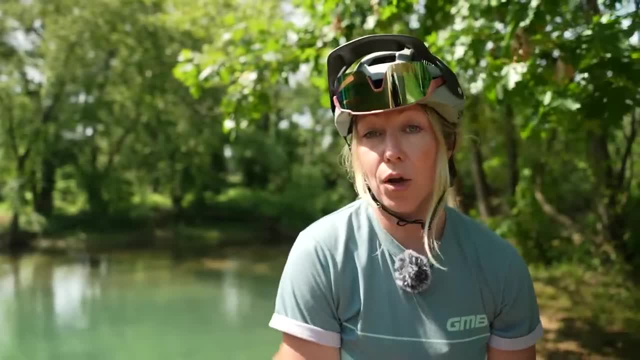 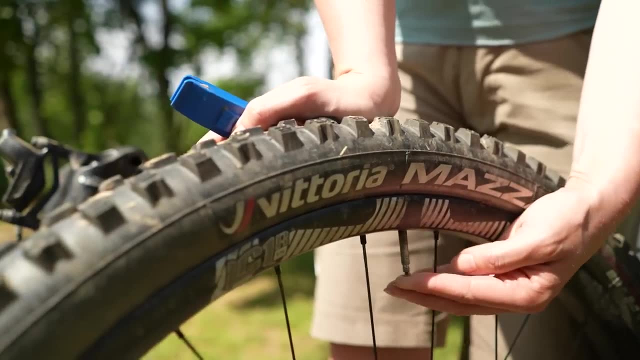 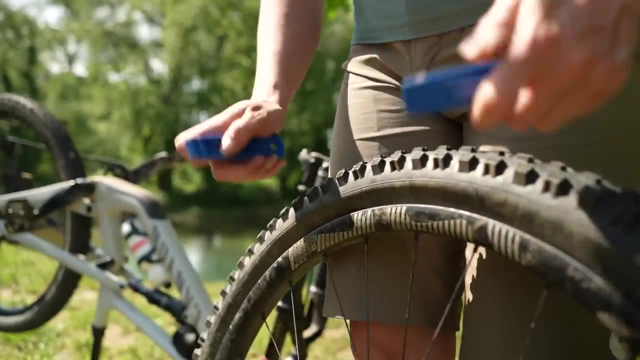 that plug and seal the hole. If that doesn't work, or if you're running tubes, then all you need to do is let out all the air- if it hasn't come out already, and use some tire levers. I recommend using with hooks on them, so that you can get two levers under the tire, and then you lever both of them. 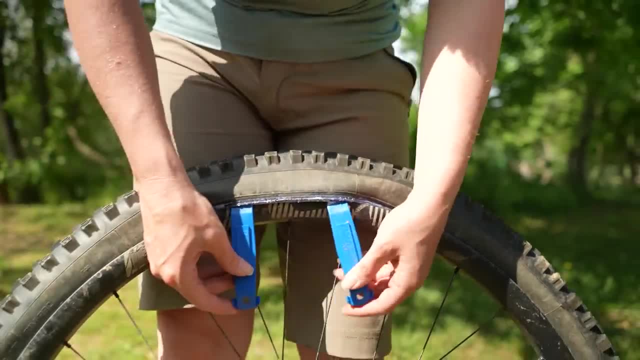 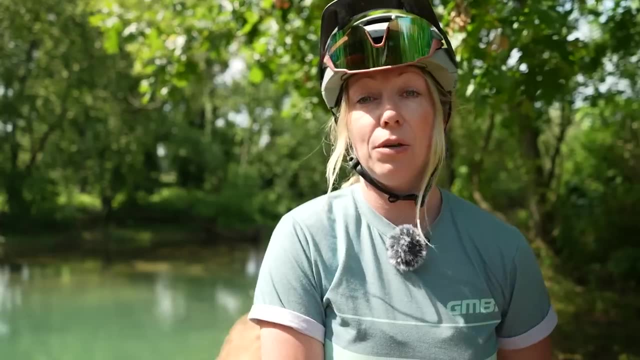 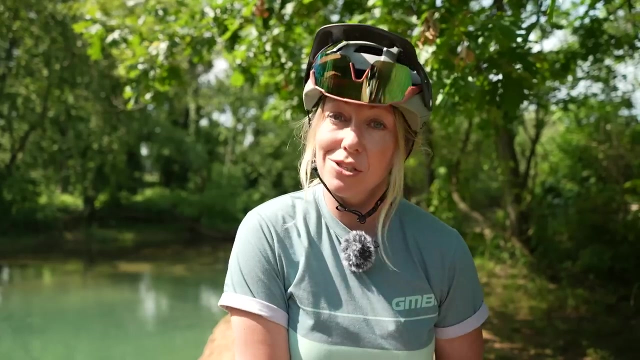 away from you and hook them into the spokes, and then you should be able to use one lever to drag it around the edge of the tire, and this way you'll be able to take your tube out or clear out some of the sealant and then put a new tube in, and all you have to do 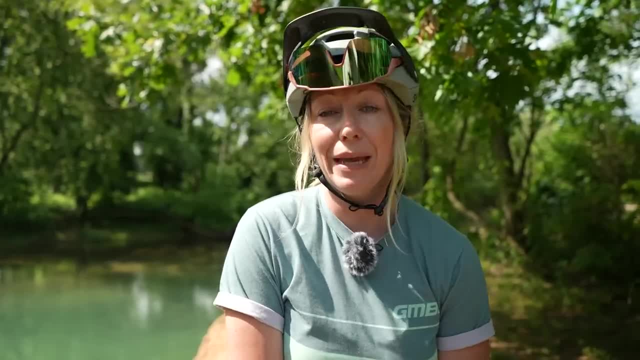 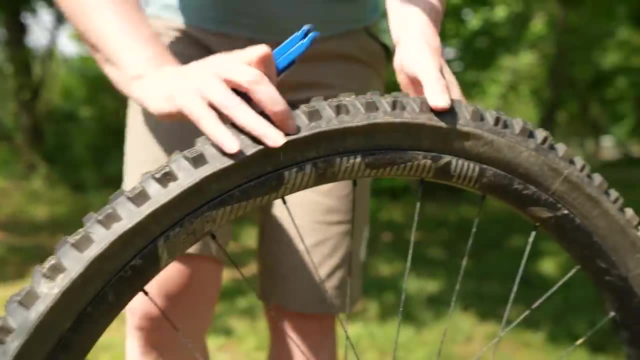 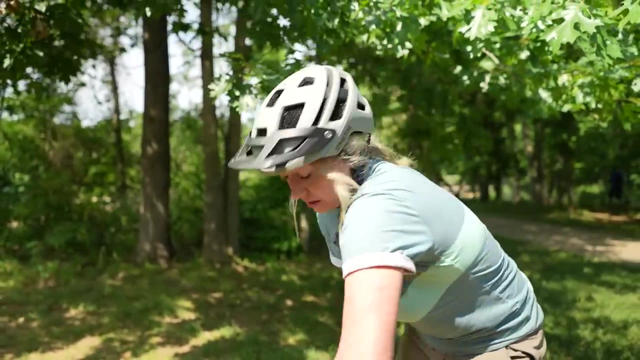 is reverse the process of popping your tire back on the bead and pumping it up. You should be good to go. it is actually much simpler than you probably think. Great bonus tip for you here if you're tubeless and your rim appears to be a little bit stuck to. 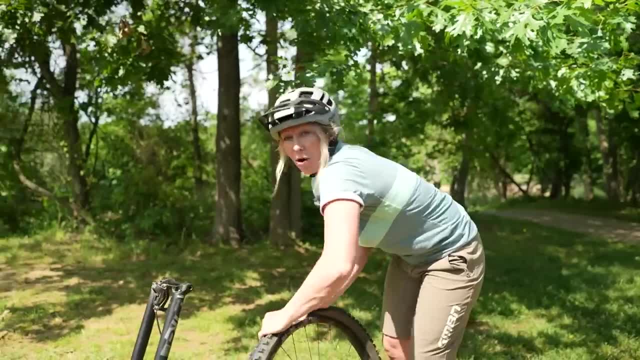 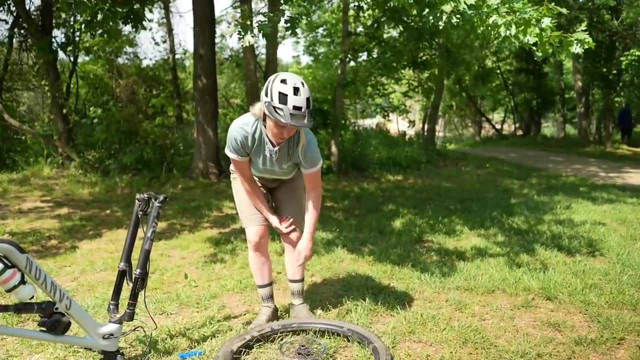 the rim and your thumb strength isn't enough to get that off the bead, then what you can do is place your wheel on the ground, preferably disc side up, so you don't contaminate it, and then you want to stand on the tire without hurting your rim. 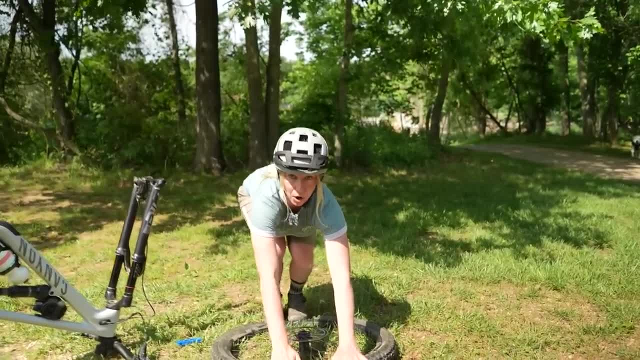 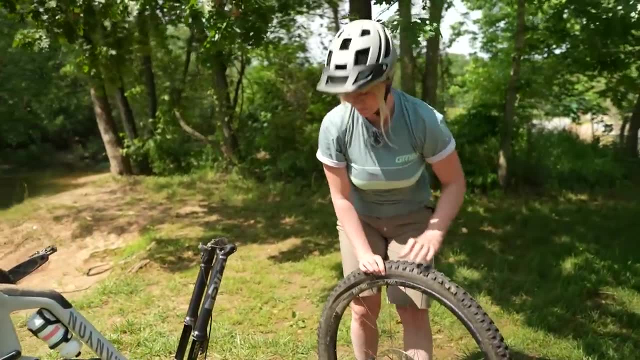 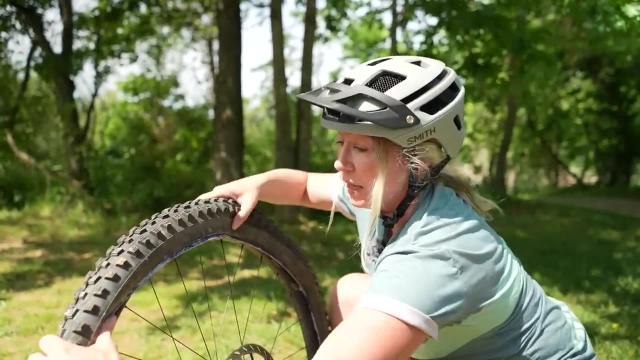 and you're going to push the opposite side of the rim to pop the tire off. There you go and then it'll come clean. simple Bonus, bonus tip is: when you put your tire on, if you just put it on the shelf of the rim, you'll get to a point where it's really, really tight and you won't be. 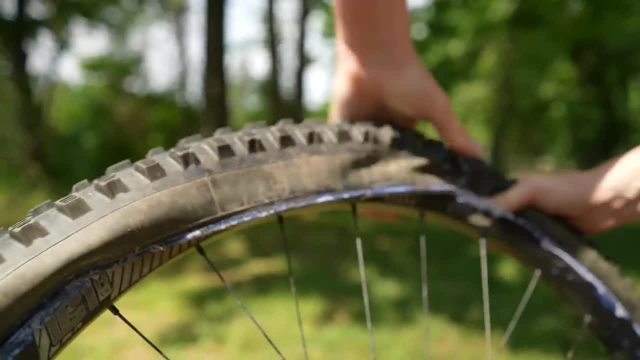 able to get the top bit on. If you move the tire all the way into the center, into that little channel, then you're actually lessening the rim. If you move the tire all the way into the center, into that little channel, then you're actually lessening the rim. 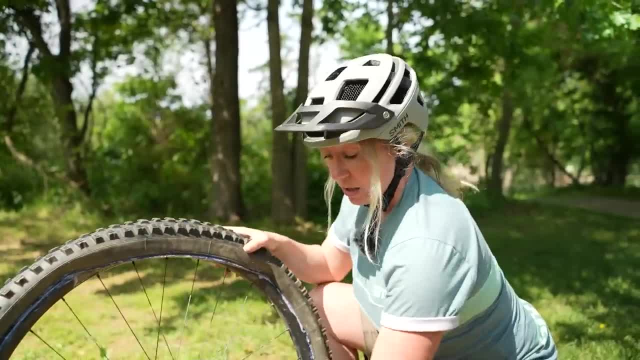 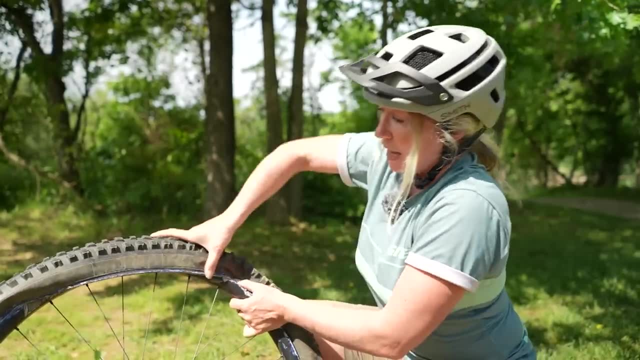 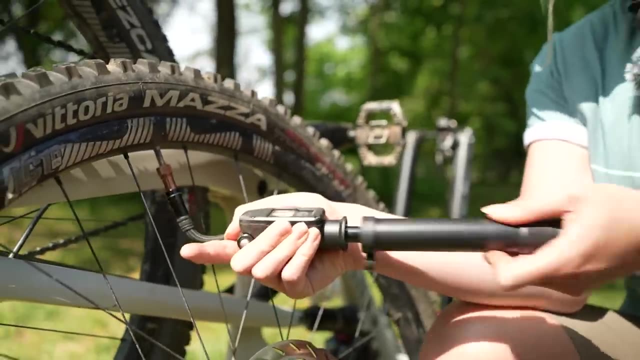 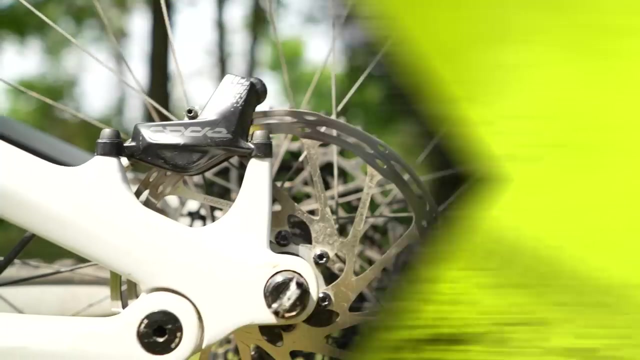 diameter that you need to push into the center of the wheel. so it'll actually be easier, and if you find that you still can't do it by hand, at least you'll only have a small bit. you'll need to do with a lever. So if you hear a noise in your desks, perhaps it's. 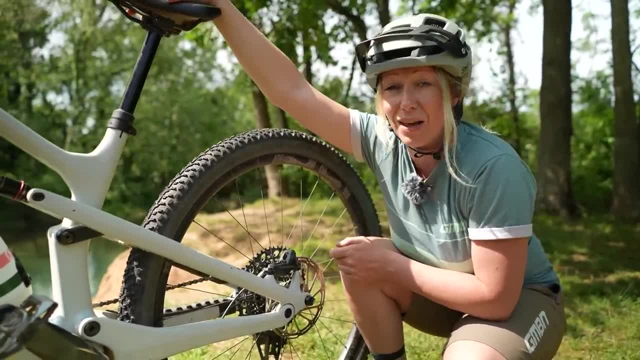 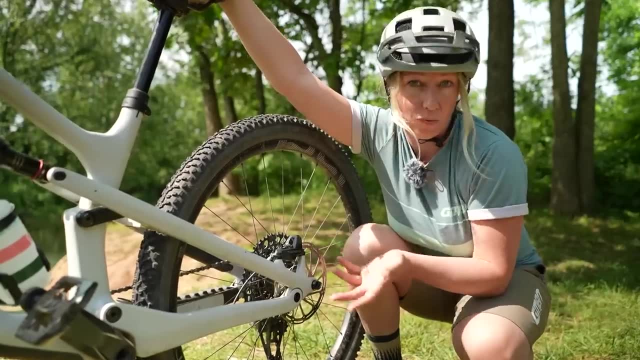 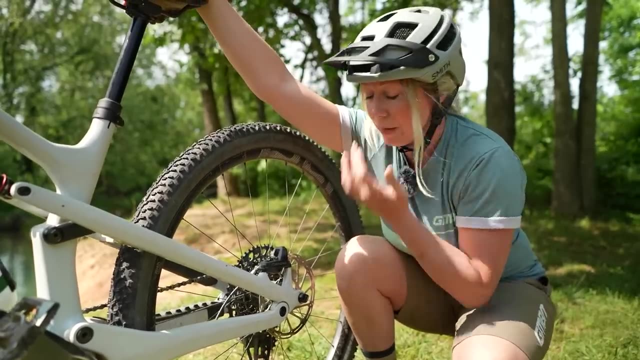 on and off, then that's possibly that you've bent your rotor and you're going to need to either invest in a rotor straightener or take it to a bike shop to be fixed or replaced. However, if you hear a constant rub and it feels like your brakes are on partly all the time, it's possible that your 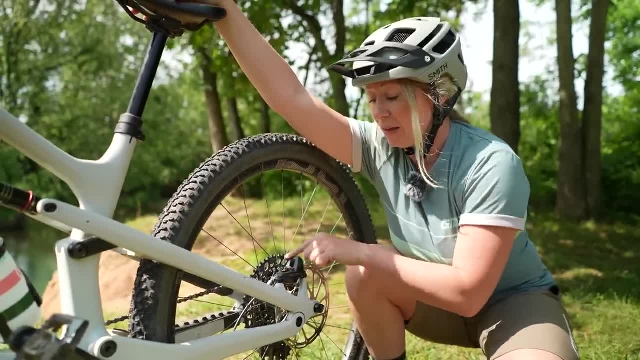 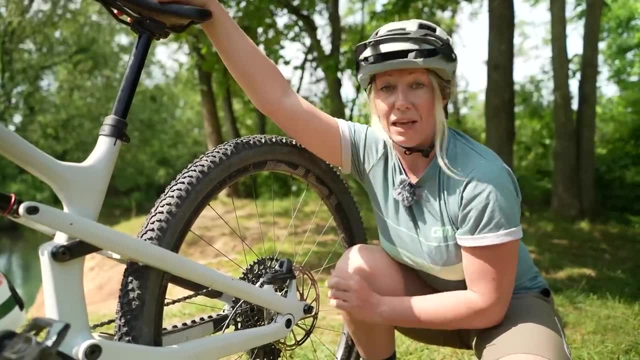 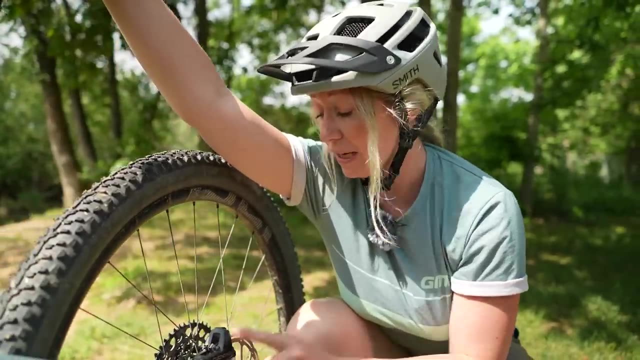 caliper is no longer aligned, so that means the pads that house inside the caliper are not perfectly or the disc is no longer perfectly in the center of your pads. This is a really easy fix. as you can see, there's two bolts that hold that caliper on, and they do move side to side independently. 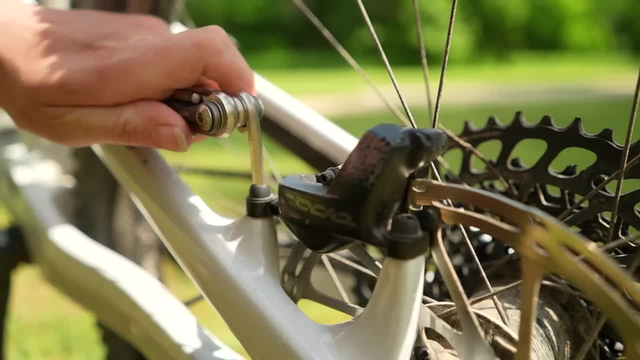 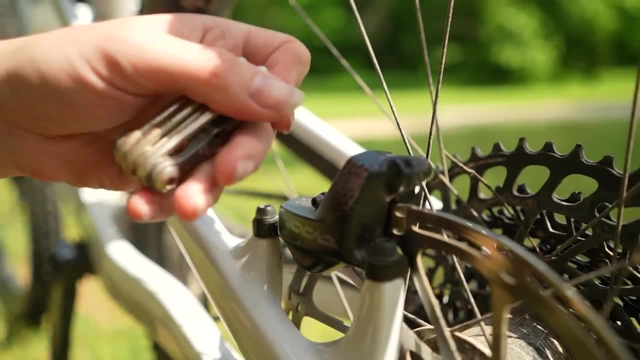 so all you need is some allen keys or a multi-tool, and you'll just want to undo them slightly so that you can move them. I personally like to have a little bit of resistance so that I don't move the caliper too much, and then what you can do is apply the correct amount of force on the caliper. 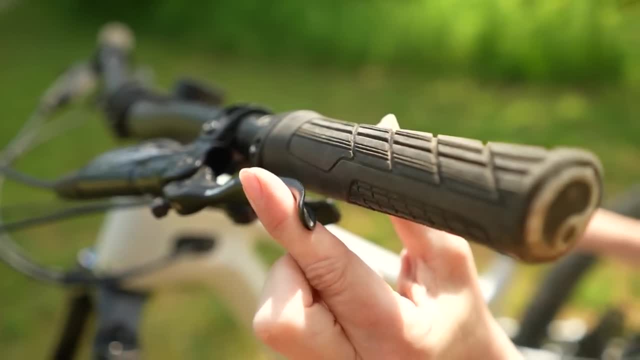 and then what you can do is apply the correct amount of force on the caliper, and then what you can do is apply the correct amount of force on the caliper brake and then tighten them up, and then that will get the disc in the center of your pads. 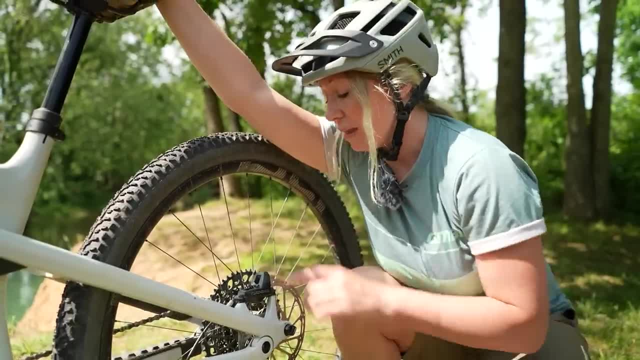 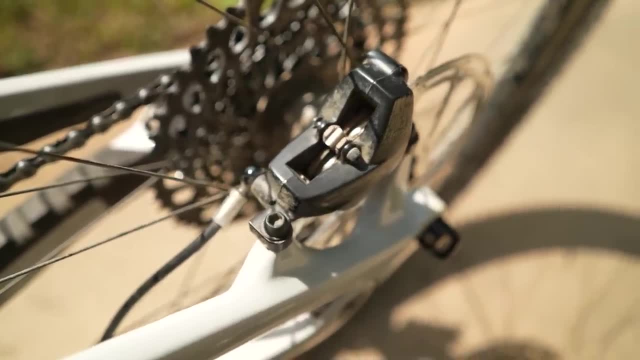 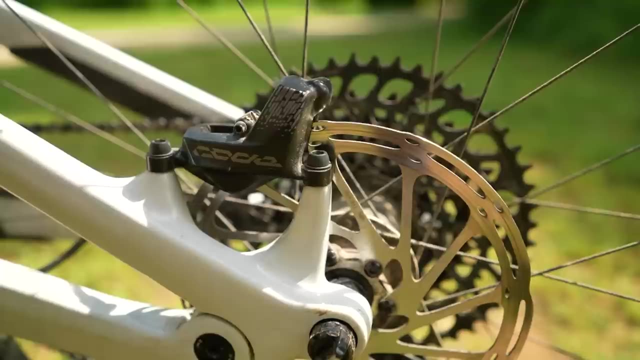 If that doesn't work, you may need to do it by eye, and this just means looking down the pads and moving the caliper until you think the disc is perfectly in the center and there's a little gap either side. but it is really simple. as long as you've got an allen key, you can do that one. 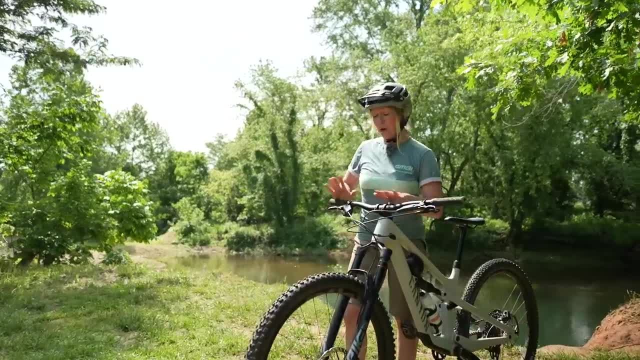 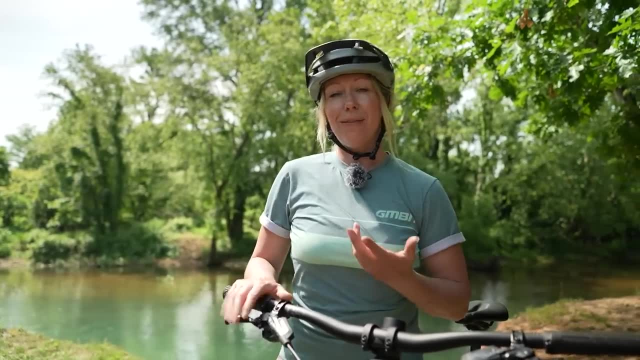 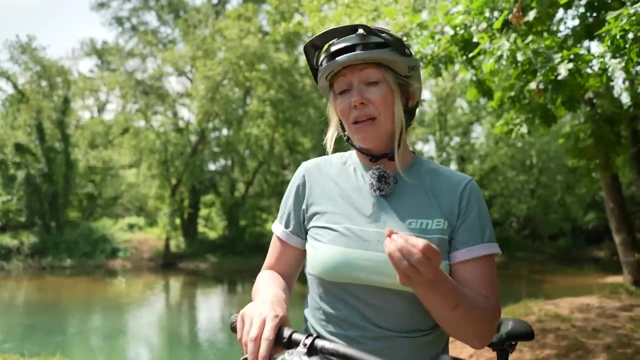 If you've recently purchased a new bike or if you've had new cables fitted to your bike, then after a week or so, or a few rides, you might find that your gears stop working well. perhaps they make a noise, perhaps they don't shift so good, and that is generally because of